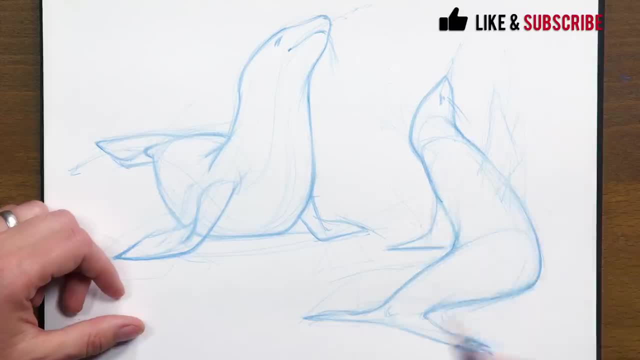 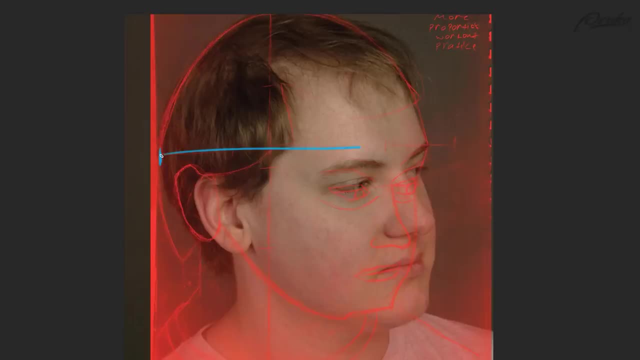 coming up, so make sure you're subscribed. As always, a bunch of these lessons are going to be free, but if you want the complete experience, with all the extended lessons, projects, demos and critique videos, you can join at any time at prokocom slash drawing. Now let's make. 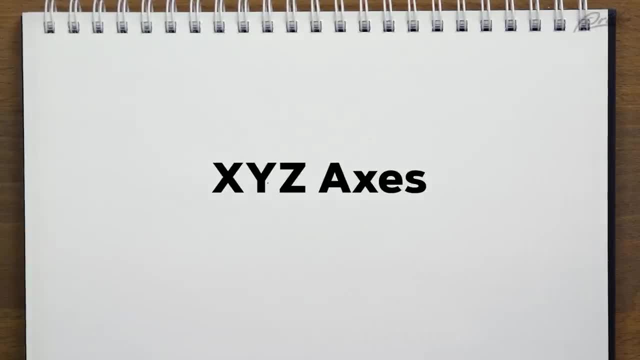 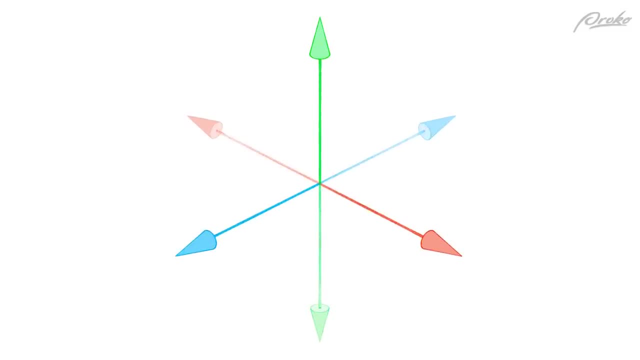 sure we understand some key concepts. XYZ axes: In 3D space we use axes to talk about directions or positions or how something is rotating. Each axis is a different dimension. The x-axis is for width, the y-axis is for height and the z-axis is for depth. They help. 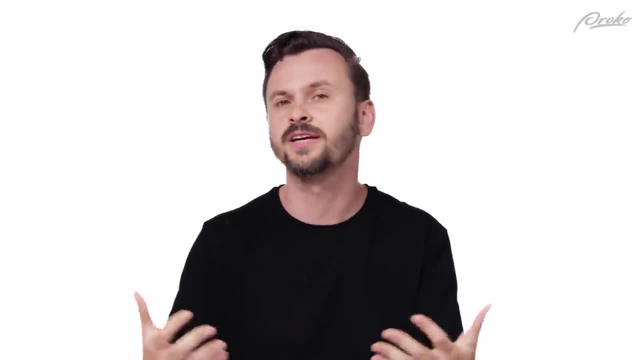 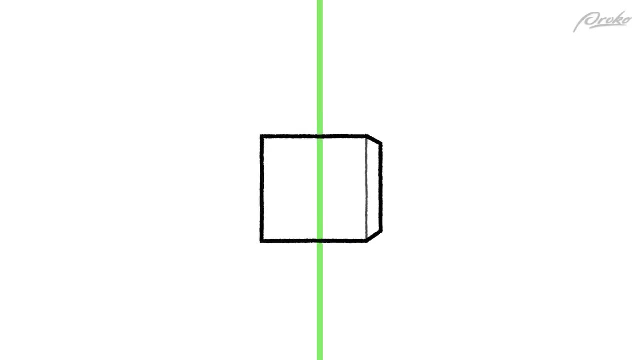 us describe what we're doing, Where something is or how it's moving in space. So if you're moving a box along the y-axis, you're lifting it up or down along this invisible line. If you rotate something around the x-axis, it's like spinning it around that horizontal line. Imagine a drill. 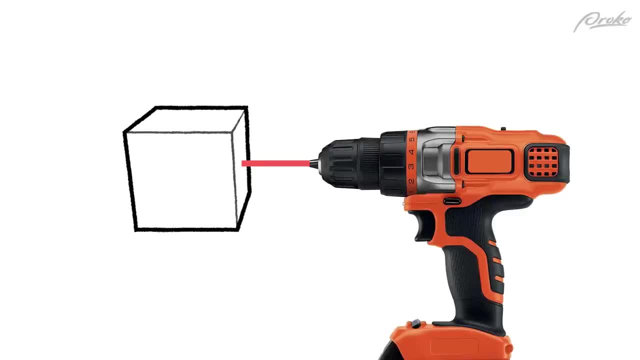 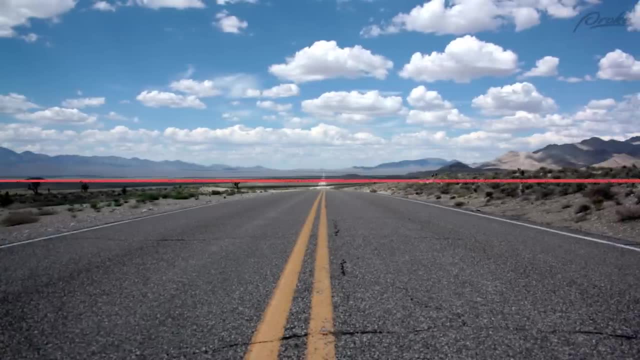 spinning in that direction. That's how the object would turn. Horizon line: The horizon line is the line where the ground plane meets the surface. The horizon line is the line where the ground plane meets the surface, The sky. This is typically the first thing you want to figure out to establish the environment. 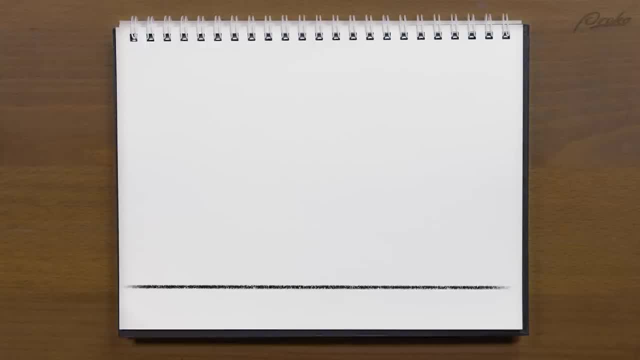 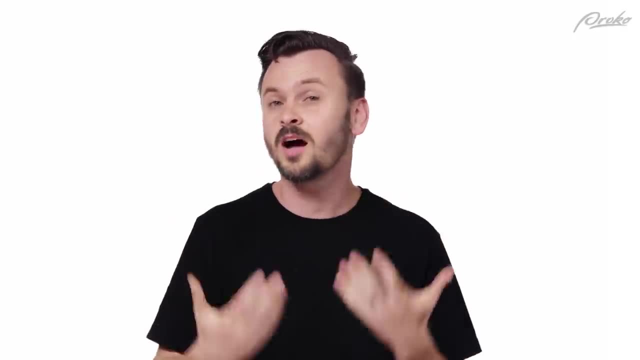 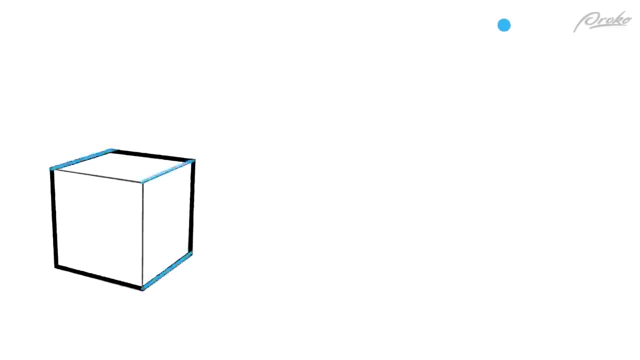 It could be anywhere on the page, Up here, down here. It could even be tilted, And this would suggest that you, the viewer, are tilted, making the composition more dynamic. Vanishing point: This is the imaginary point where all the edges of one of the axes on a box converge. 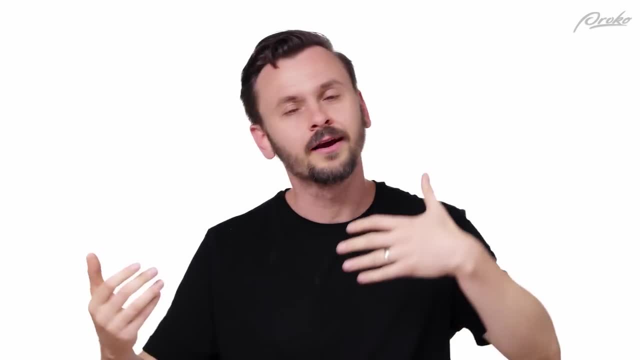 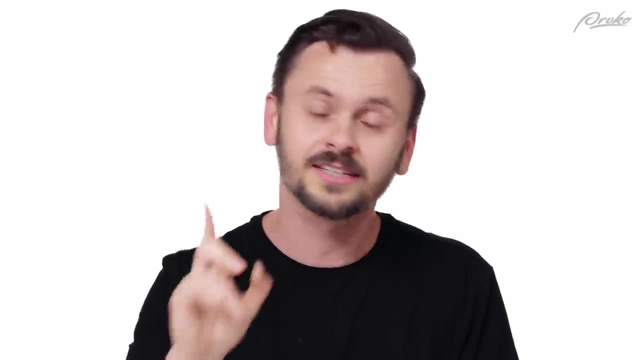 A drawing can have one vanishing point, two, three, five vanishing points, even 27 vanishing points. You can have as many as you want. We're gonna stick to one today And for a while we're gonna keep our vanishing points. 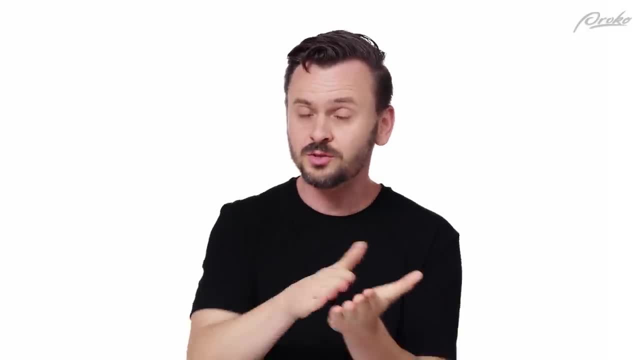 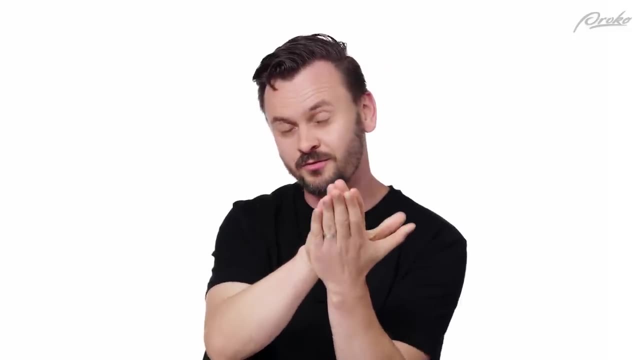 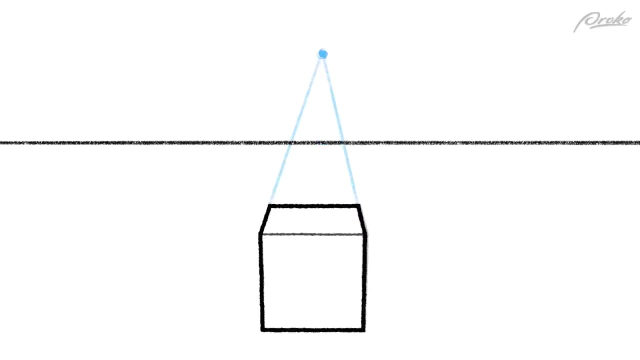 on the horizon line. Just keep in mind that as soon as we rotate something up or down, that thing is no longer parallel to the ground, And so the vanishing point will no longer be on the horizon, because the axis is no longer pointing at the horizon. 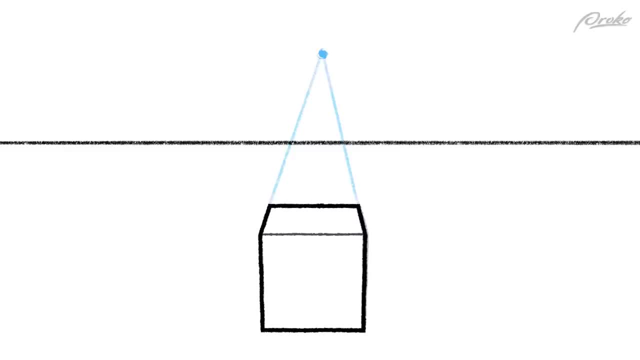 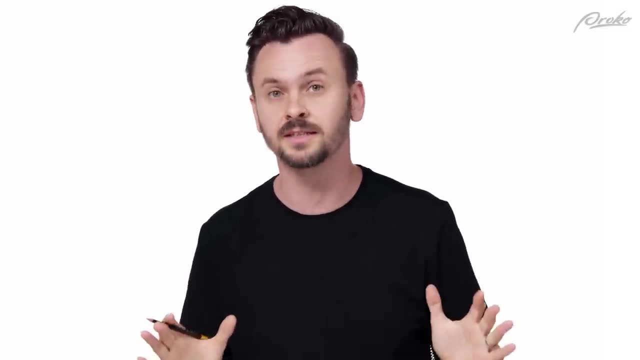 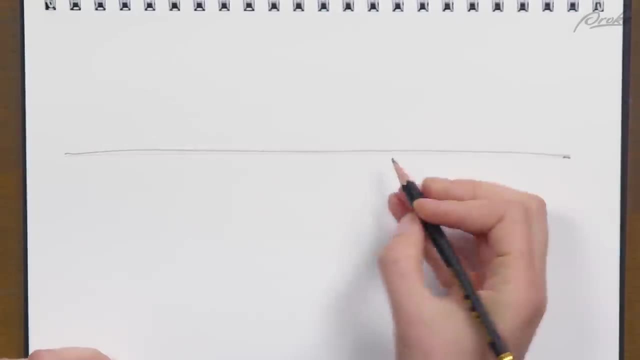 So a vanishing point represents where, in the distance, the axis is pointing. All right, So let's sketch a simple one-point perspective scene. I'm gonna start with the horizon line, just a simple horizontal line, And I'm gonna put a 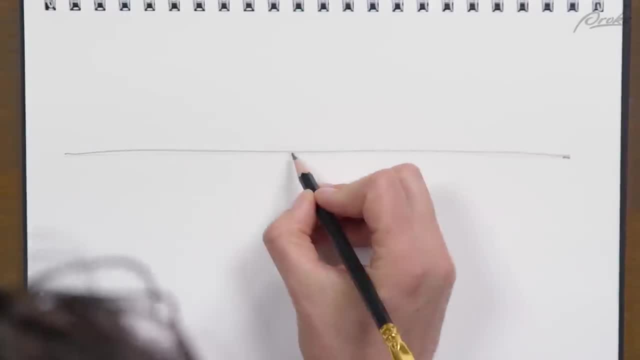 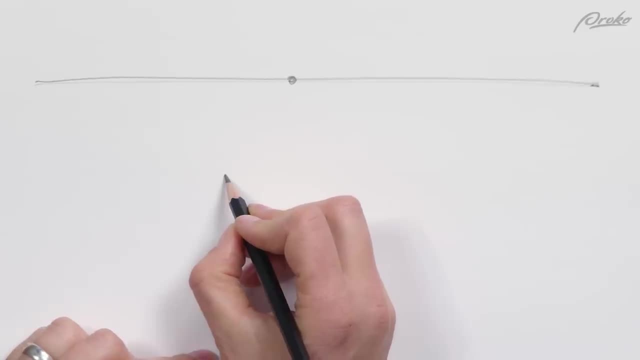 vanishing point, single vanishing point, somewhere along that horizon. Just do it right there. The first step for drawing that box is to figure out that front-facing plane. So I'm gonna start with a simple rectangle below the vanishing point. So at this point it's just a rectangle, It's not. 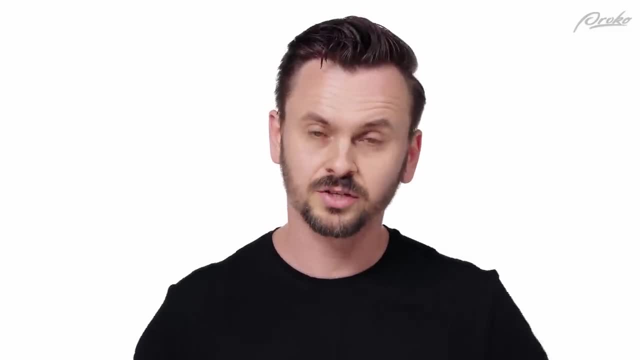 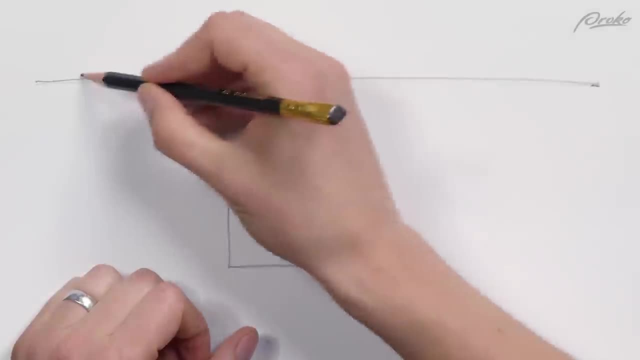 a three-dimensional form. In order to make it three-dimensional, we have to extrude it, we have to give it some depth And because this is a one-point perspective scene, we have to extrude everything towards that one point. So this box is below the horizon line. 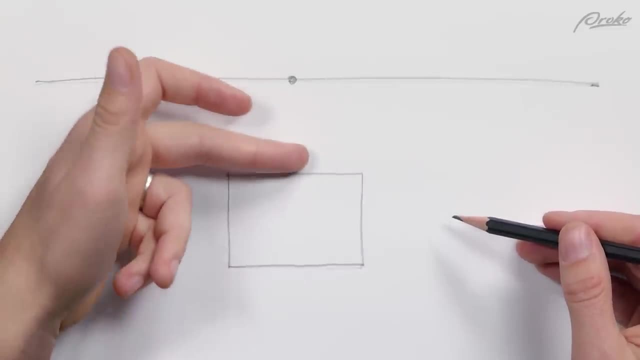 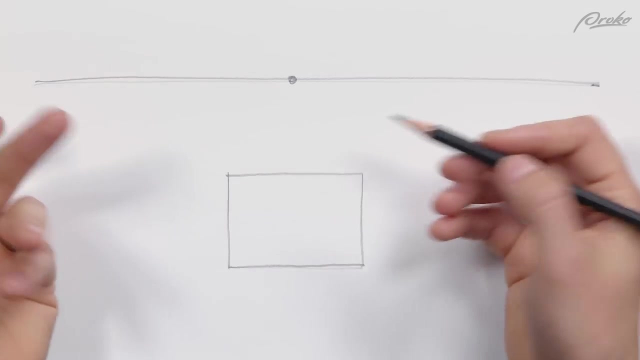 which means we're looking down at it and we're going to see the top plane. If it was above the the horizon, we'd be looking up at it and we would see the bottom of it. So with this one we're seeing the top. so let's extrude that top lane towards the vanishing. 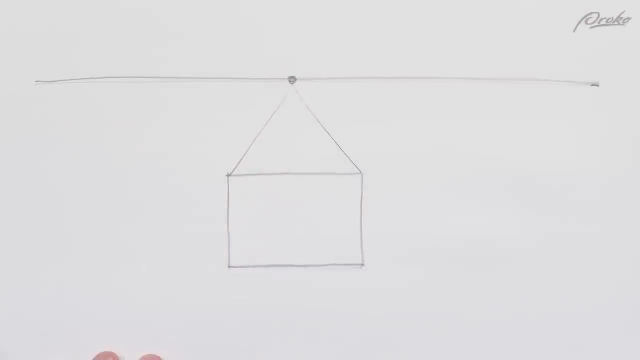 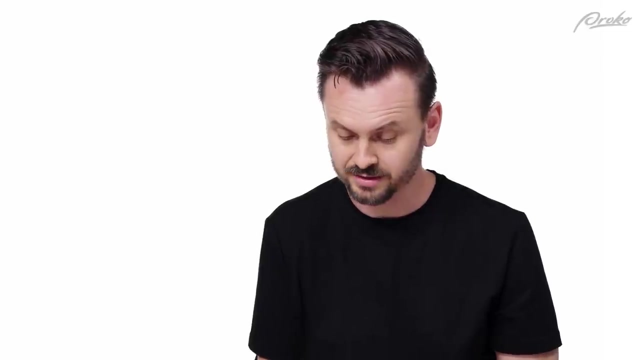 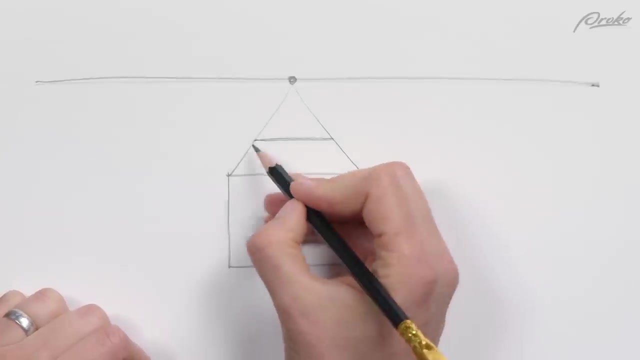 point like that. And so now we have this box that just keeps going forever into the distance. it never really ends. If we want to end it at some point, we could cap it off. just add a horizontal line, say there's that back edge. 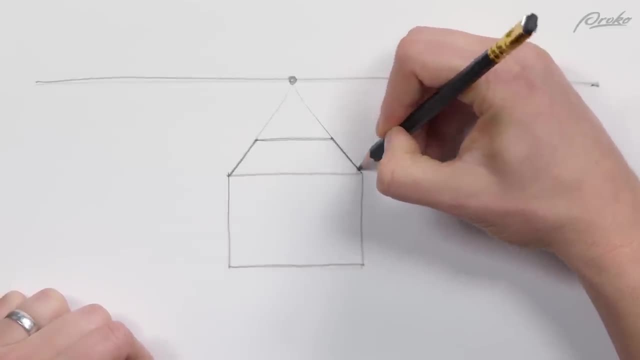 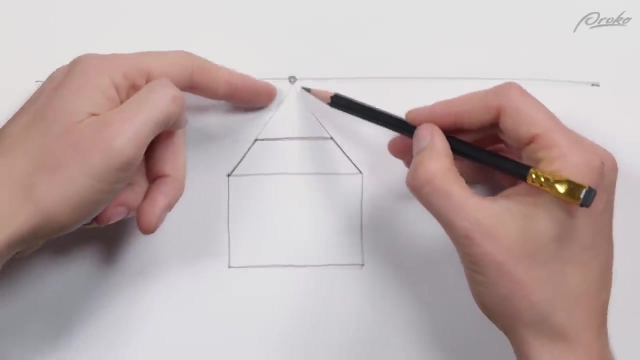 Once we establish the back edge now we know it ends there. but those lines still converge, they keep going. even if I didn't draw them all the way to the point, They're still converging towards the point. they just end before they go all the way to. 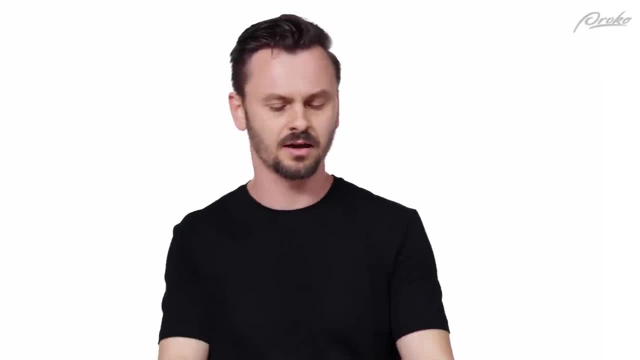 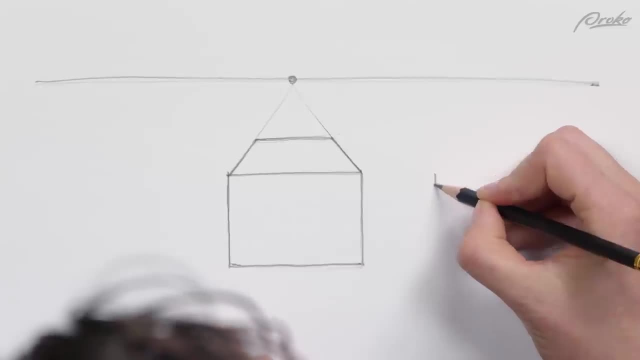 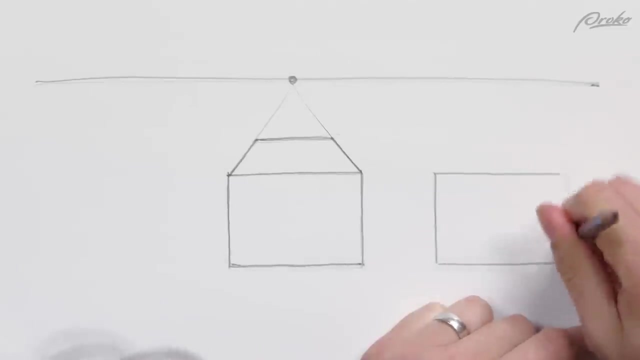 the distance. So what if we wanted to have this box off to the side, not directly below the vanishing point? Well, let's try it. So all we do is we just draw another rectangle Off to the side and extrude these lines: 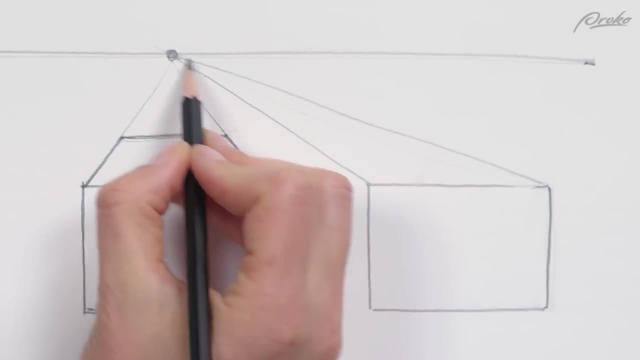 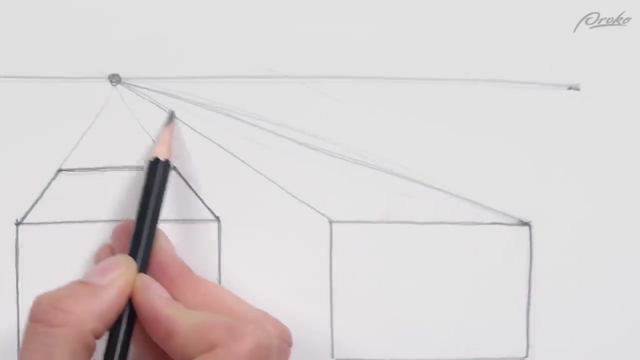 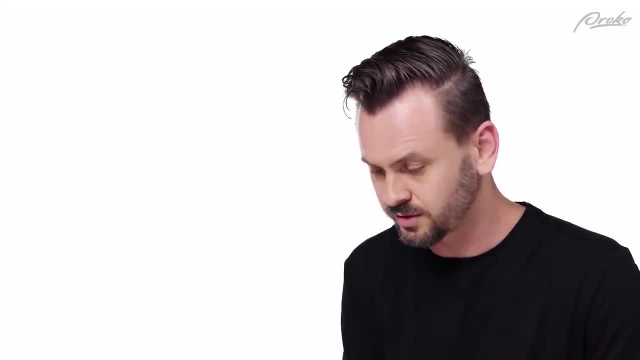 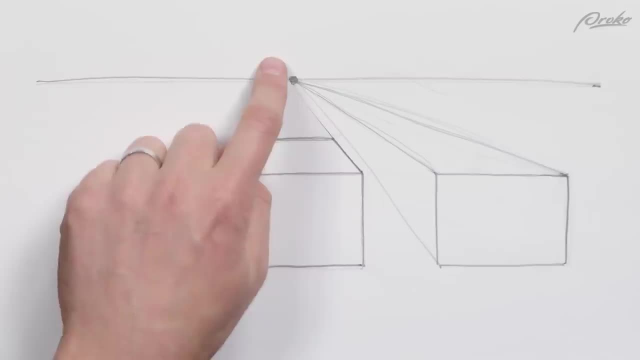 Yeah, Yeah, Drawing lines from point to point. If you haven't been practicing that one, maybe you should start including that in your warm-ups as you prepare for more perspective assignments. Now notice, I have a third line here, the bottom one. 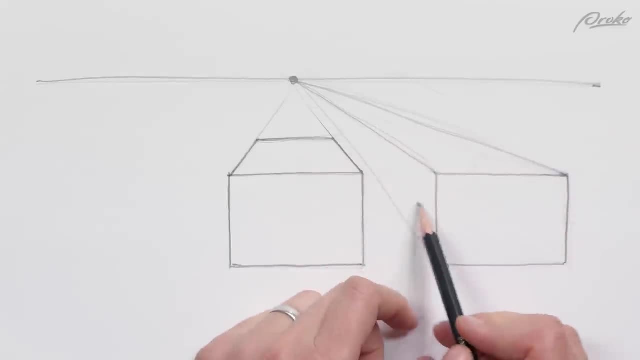 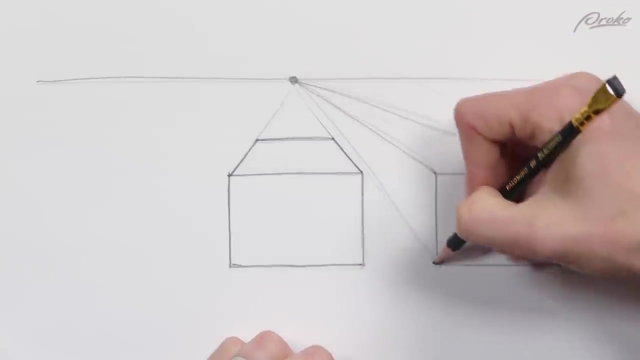 Since we're now shifting this over to the side, we're going to start seeing the side plane a little bit, not just the top plane, and so we added one more corner, converging, And when we cap these off we draw that back top edge over here and from that same corner. 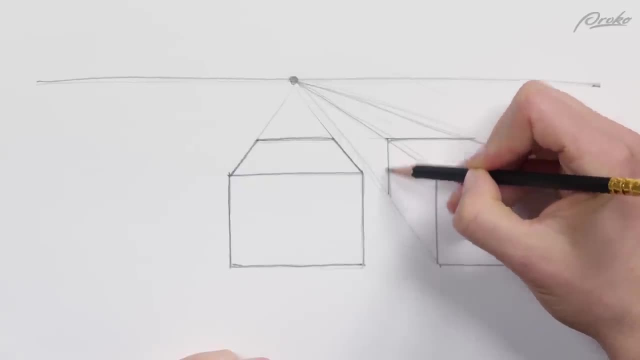 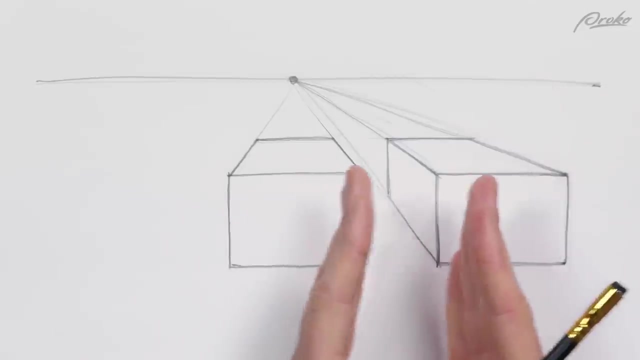 over here we can drop a vertical line and that is the back edge of this side plane. now, Okay, there you go. So now you have these two boxes side by side. This one is not rotating, it's just shifted over to the side. 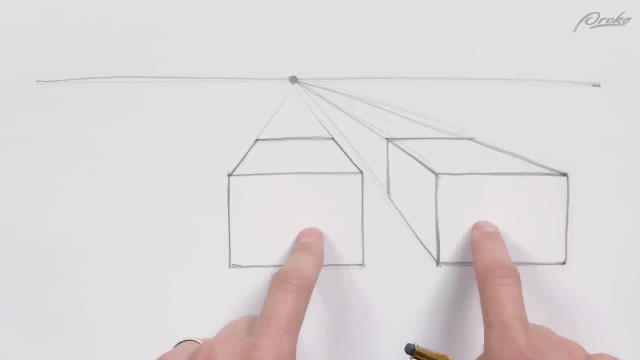 And the reason that we know they're not rotated is because these front planes are both facing the same direction. right, We're seeing the flat part of both. If we were to actually rotate this one, it would not be perfectly vertical and horizontal anymore. 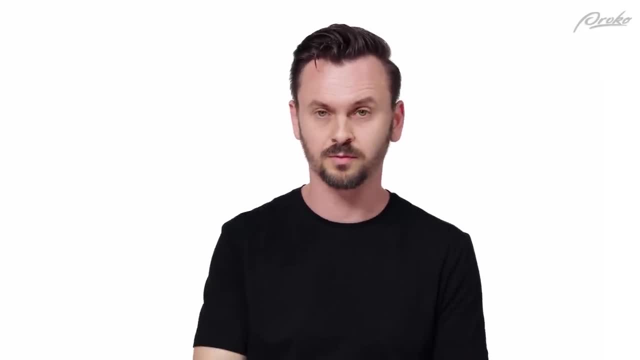 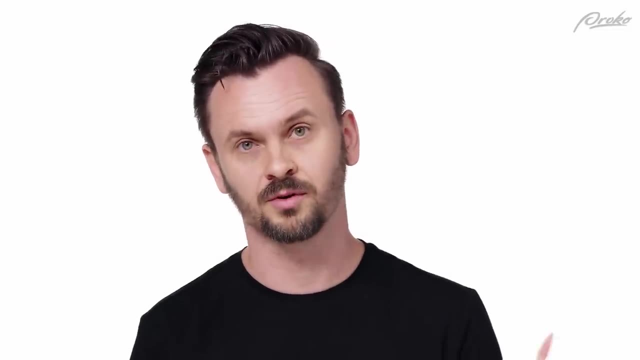 And so that's one really important rule for one point perspective is that these front planes, they kind of have to face us, Otherwise we'd need to add more vanishing points to accommodate For these other lines. Now let's do another one. 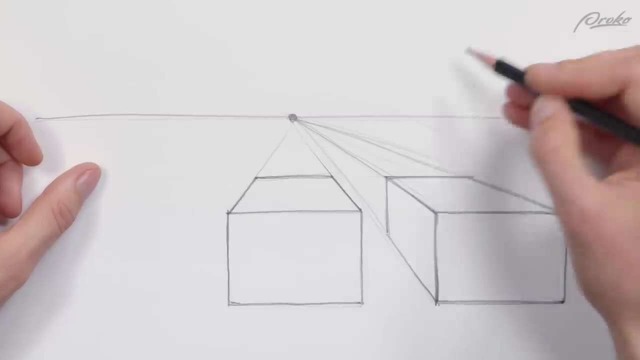 Let's do a box right on the horizon line, like passing through the horizon. So let's say it's right there, that rectangle. Now we're not below or above this box and so we're not going to see the bottom or the. 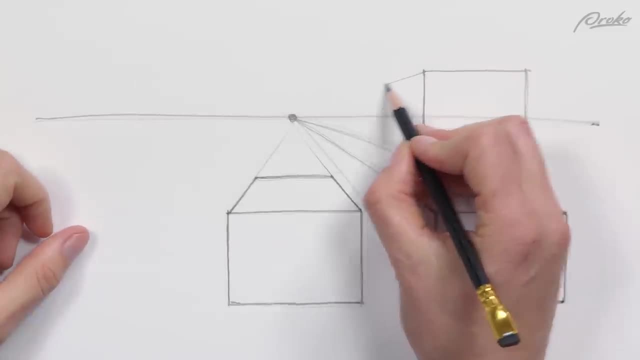 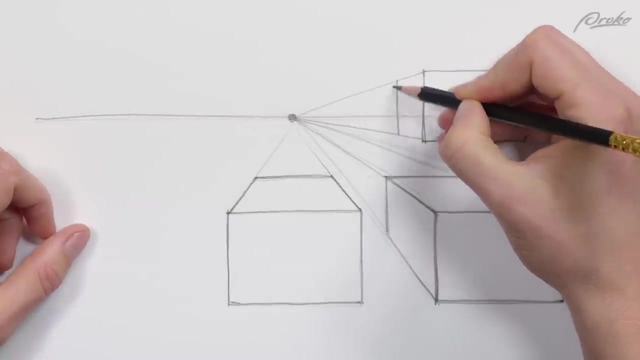 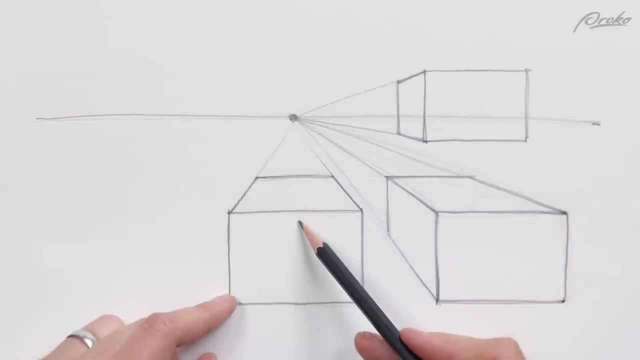 top plane. Instead, we have to project this, So we're not going to see the bottom or the top plane. Instead, we have to project this. So we're going to see these corners and we get a side plane. So it's the same as this box here, it's just that now, instead of being directly below, 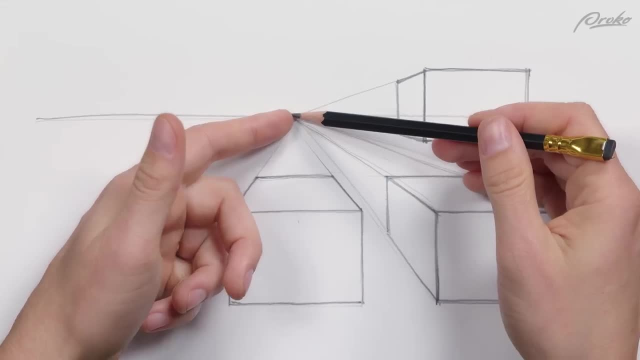 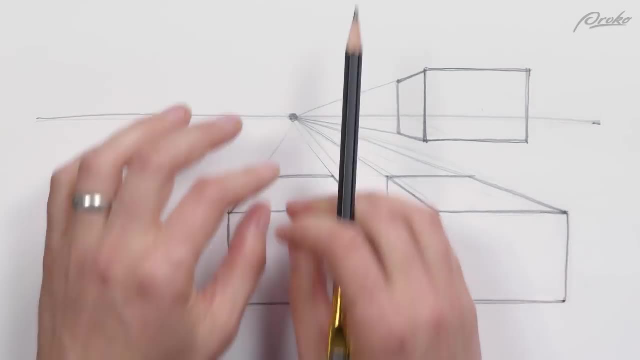 it's directly to the right. So anytime a box is directly below, to the right, above or to the left, we're only going to see two of the planes. If it's kind of offset from that, Then you're going to see three planes. 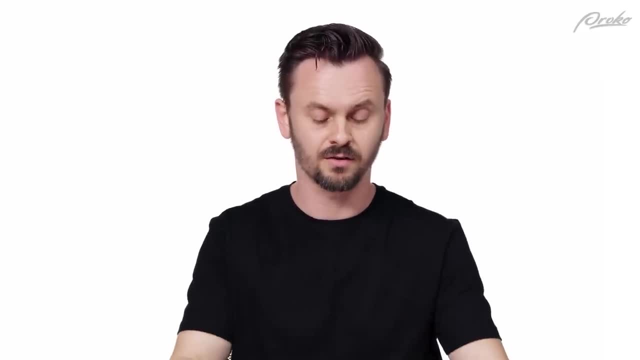 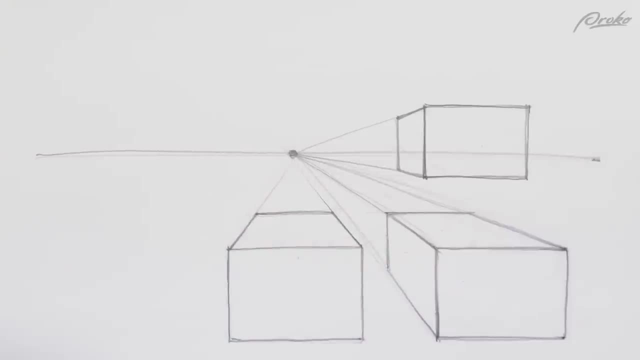 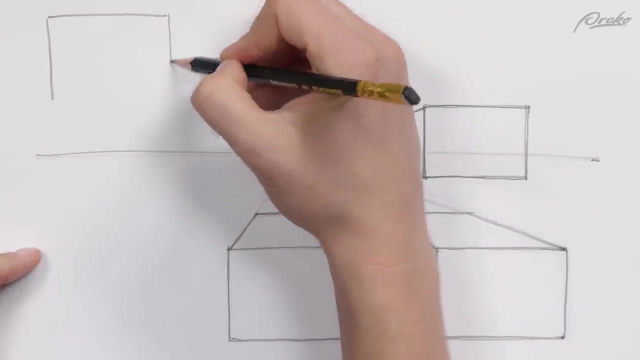 Okay, now let's do one more and let's put it above the horizon, So as if this box is floating up in the sky, or maybe attached to the ceiling, some kind of air conditioning unit or something. So we'll start with a rectangle, just vertical and horizontal lines. 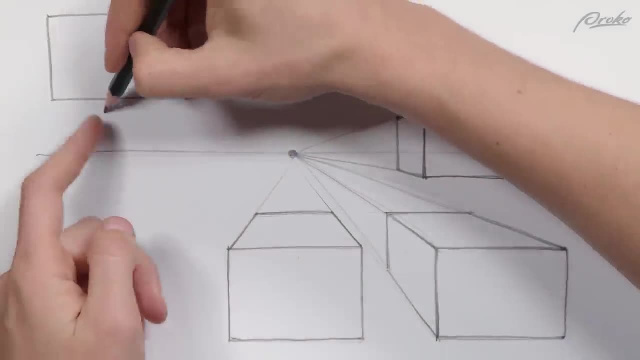 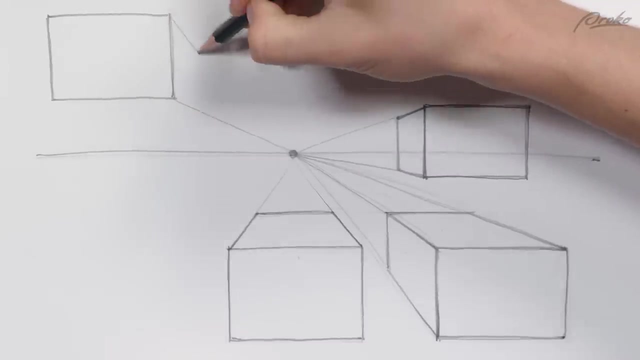 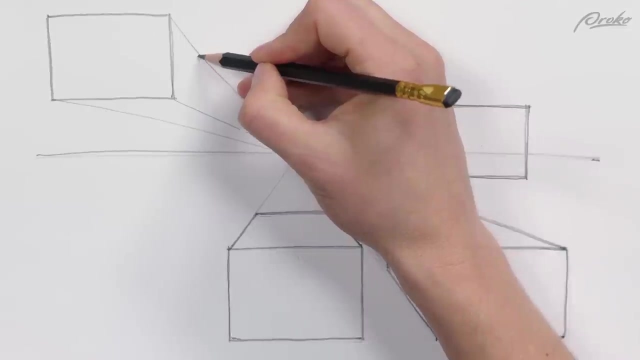 We're looking up and to the left, and so the bottom and the right planes are going to be visible. We can see some of those. We're going to go over here, So I'm going to zoom in and just tap this off wherever I feel like it. 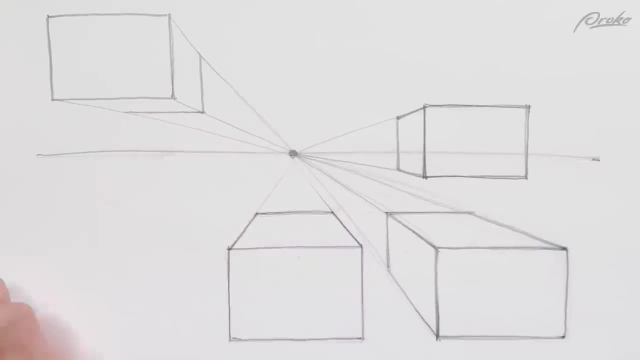 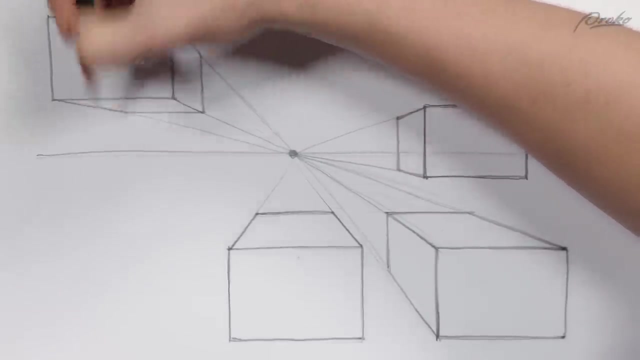 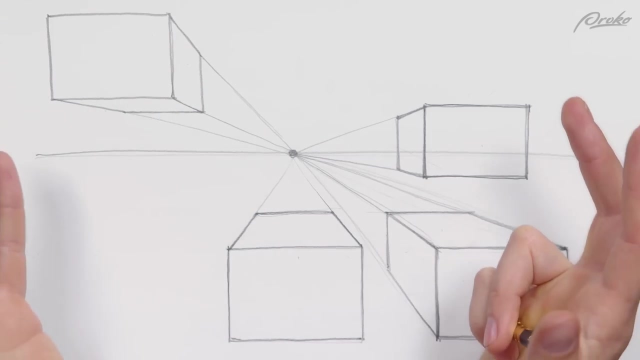 So there you go. Now you have a little bit of a hole in the sky. Okay, now let's see the top. So there you go. now you have four boxes in the same environment. they're all parallel to each other. 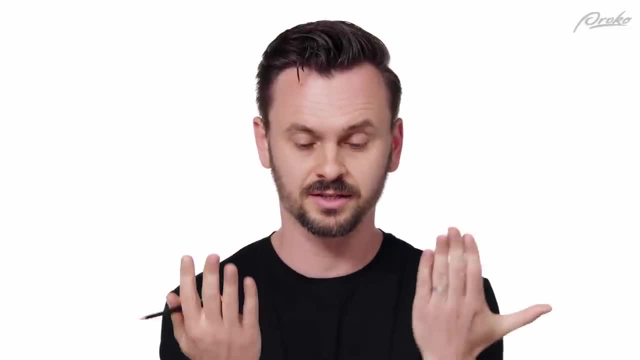 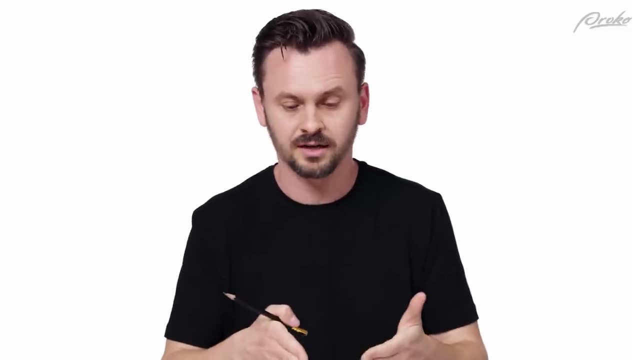 So the front faces are all pointing directly at us, or not directly at us, directly at the plane that is parallel to us, and none of them are rotated. they're all just kind of shifted to the left, to the right, up or down. 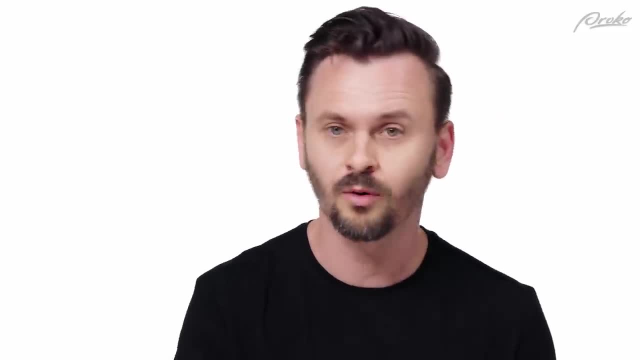 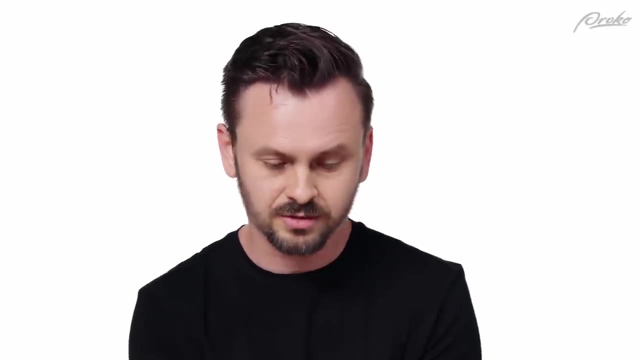 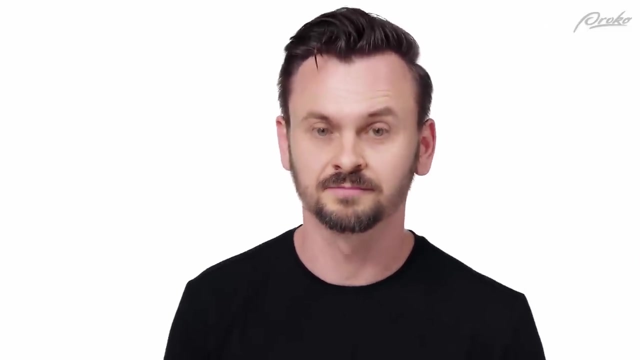 So it's not too hard. you just as long as you have one point somewhere and you can create circles. you can then extend those correct corners out to that vanishing point, cap them off and you can get boxes anywhere you want in that scene. 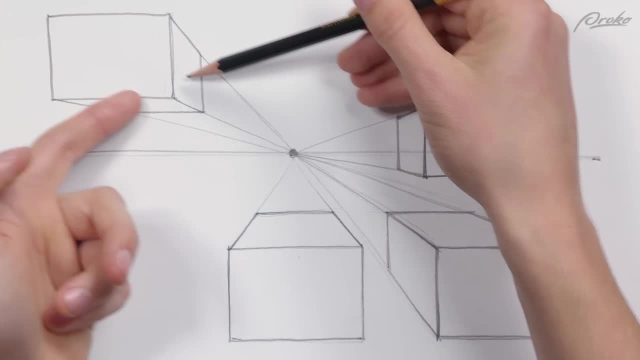 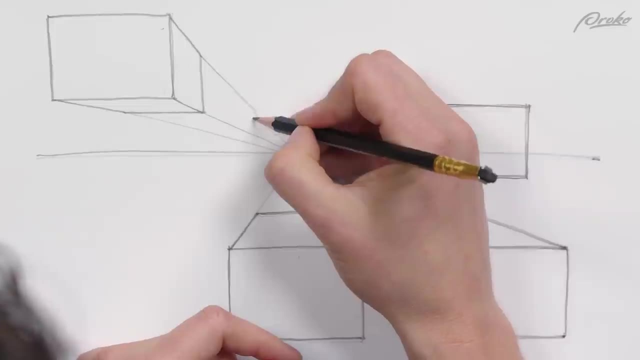 I could say: what if I want to make this box just move back into space? Well, I could just say, okay. well, it's the exact same box, I'm moving it that way, so let's just put it somewhere farther away. 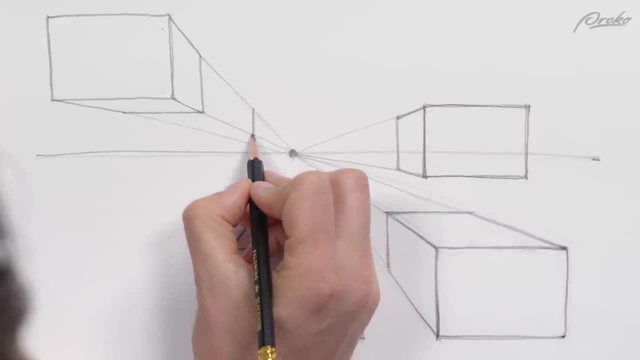 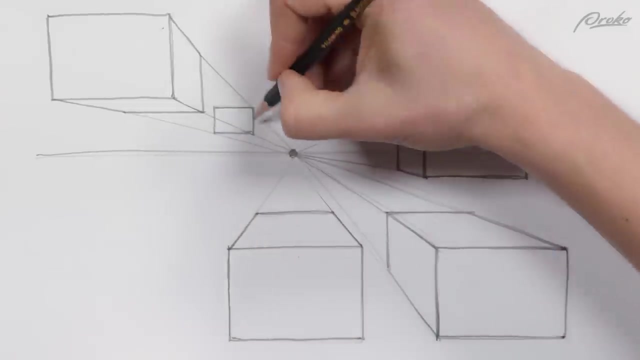 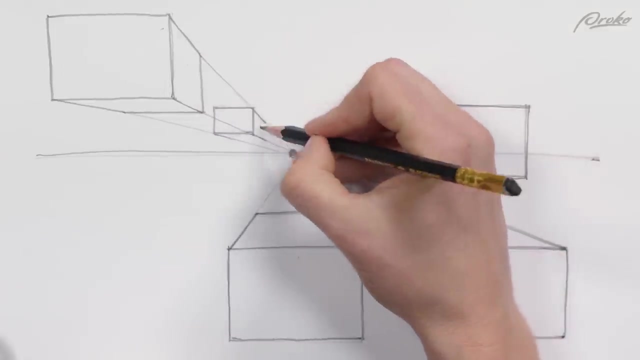 I'm going to put it here. So there's that same rectangle, just smaller because it's farther away. There's your diminution, Same convergence towards the vanishing point, And then you know there are mathematical rules of you know figuring out where to 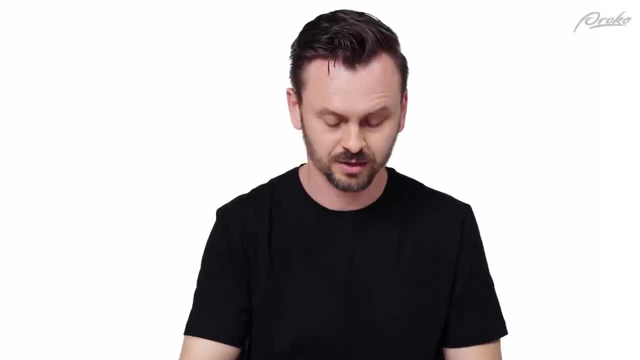 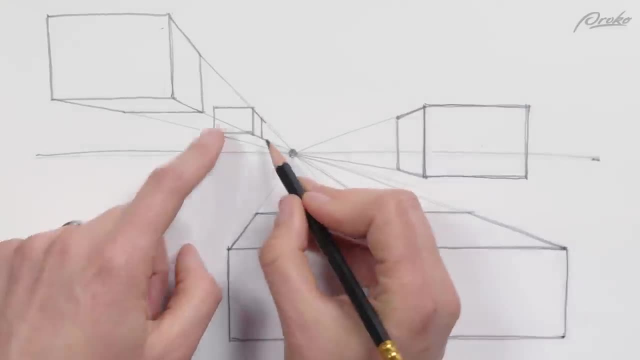 cap it off to make it exactly equal to this. that's a little too complicated for now, so let's just do it. But by eye let's say it's somewhere like this that looks like it's the same relationship between side plane and front plane. 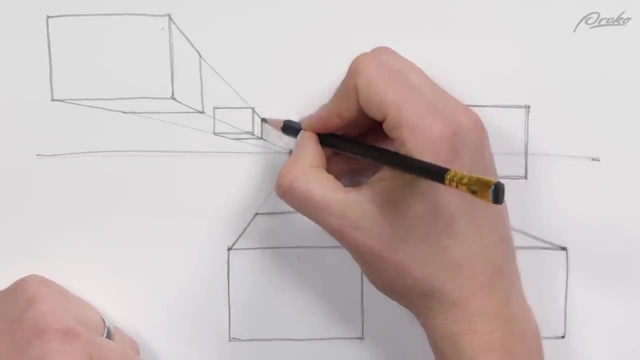 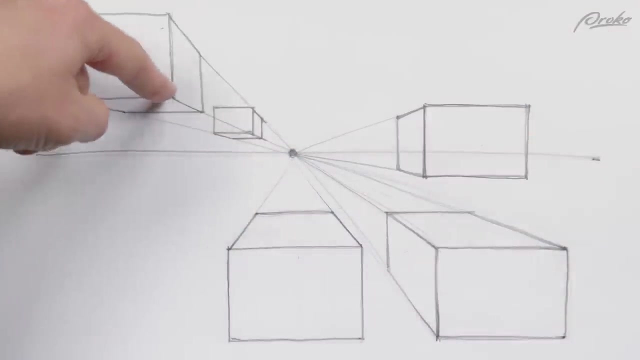 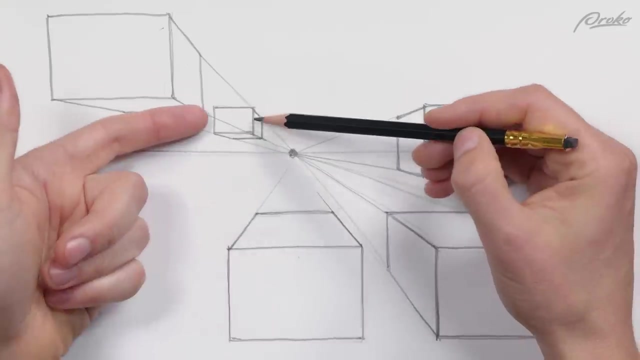 It's close enough for us to be to communicate what we're trying to communicate. So there you go. As long as we're following those lines, we are pushing that box directly away from our plane. And if I wanted to move it up or down. 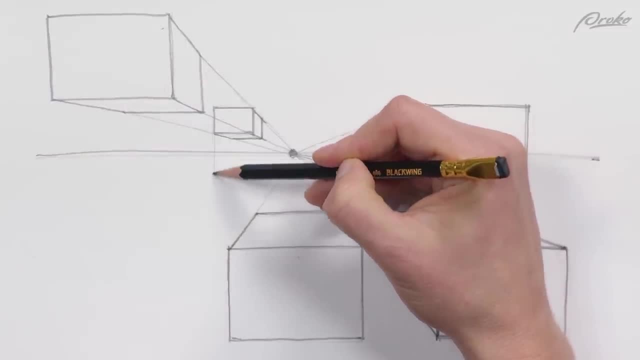 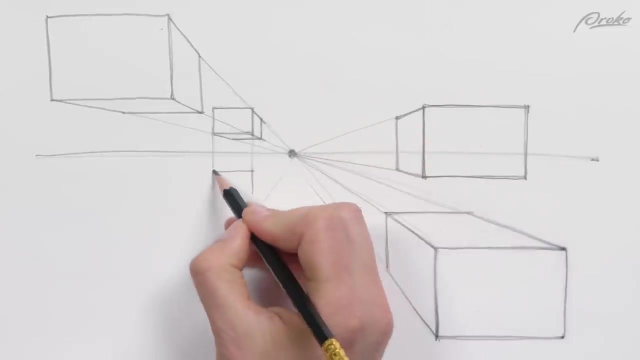 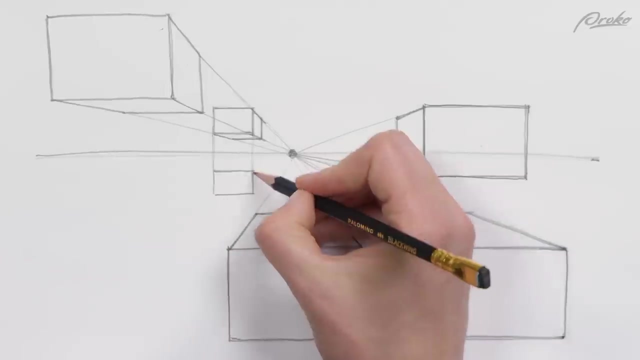 Up or down, or left or right. I just drop a vertical. so I'm just moving this same box downward and I'm just gonna Now, based off of this width, I'm gonna eyeball the ratio of the width to height. Again, this is just I'm eyeballing that. you can, of course, measure that with perfect. 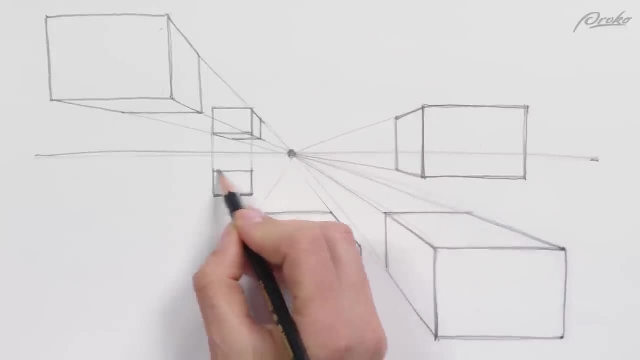 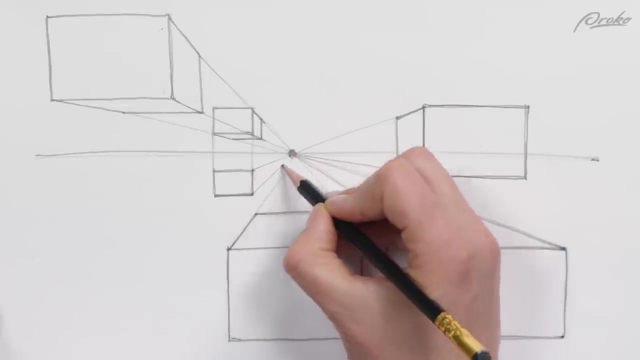 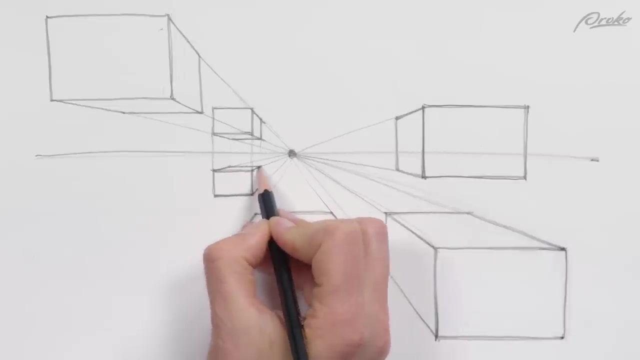 math, But So I'm going to eyeball it and make it a little bit too skinny. but you get the point. And then from there, now we can just project it the same as we did with all the others. This one drops down as well, and there you go. 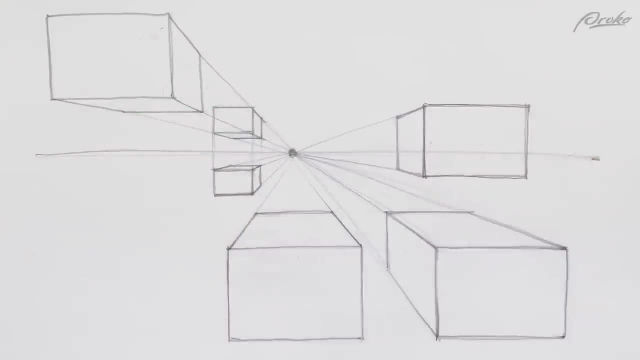 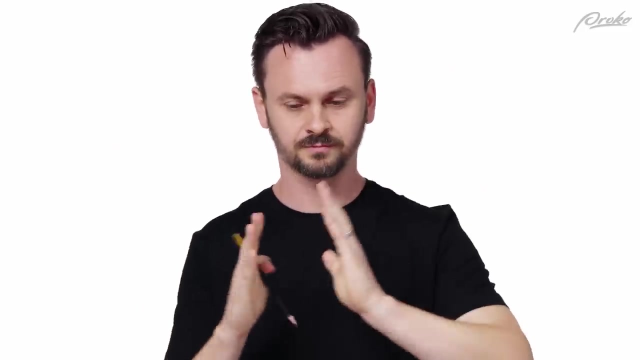 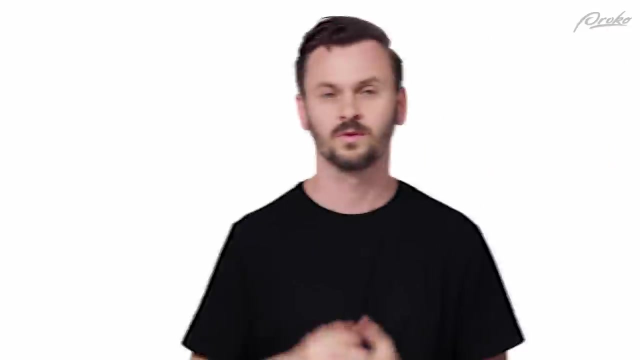 Now we have this box going into the distance and down, So It's not too hard to just. you got a box and you want to move it left, right up down. One point: perspective is a great tool for this. Limitations of one point. 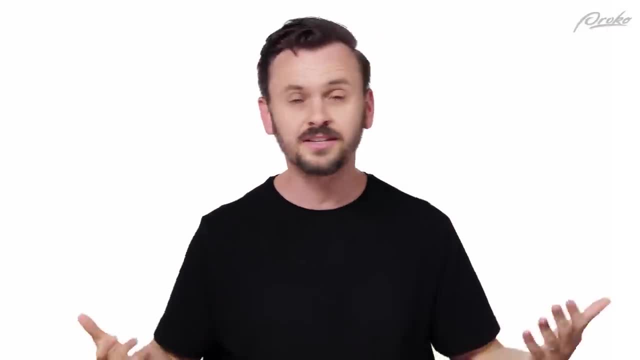 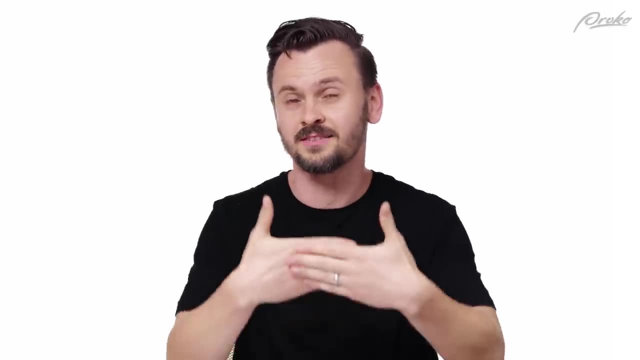 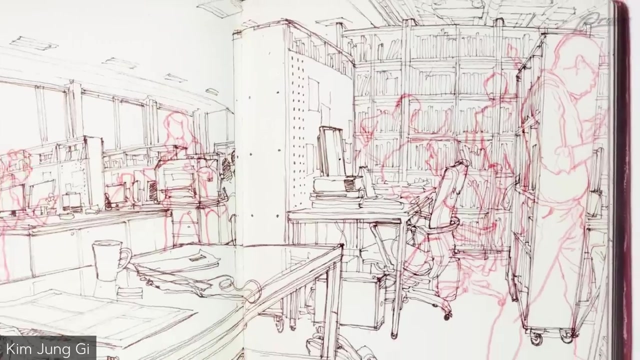 One point perspective is very simple. it's easy to use but it's very limited because the front plane of that box always has to face the viewer. It's commonly used for room interiors. when the camera is directly facing a wall, All the furniture, assuming it's parallel to the walls, will go to that one, vanishing. 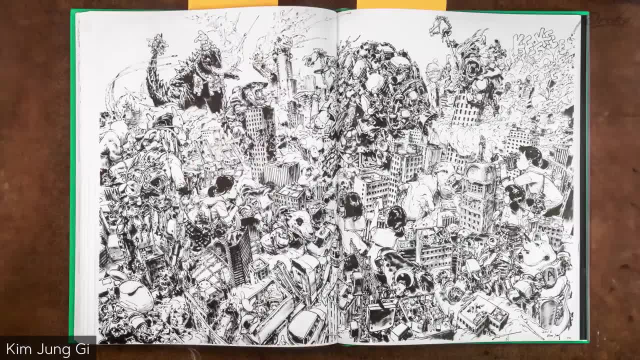 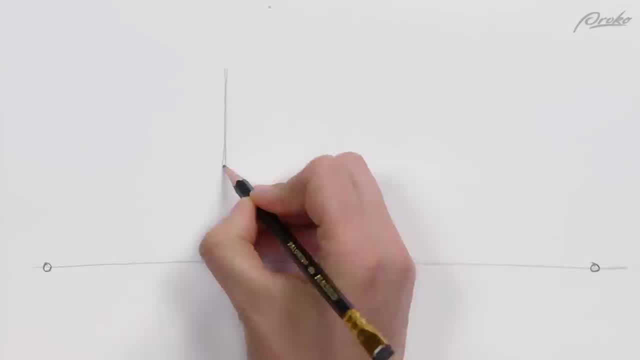 point. But when we draw complex scenes with characters and props, it's unnatural for everything to face the viewer perfectly As soon as we turn a box in space. we now have not one but two sets of lines converging to two different vanishing points. 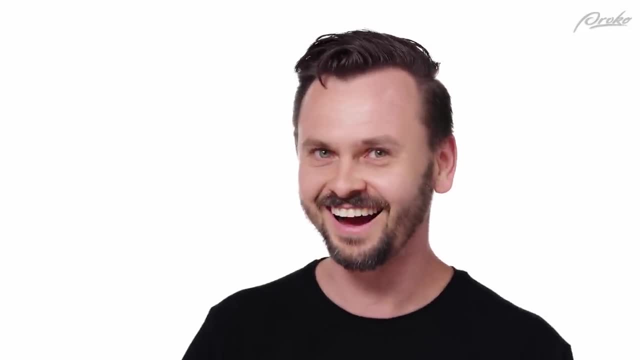 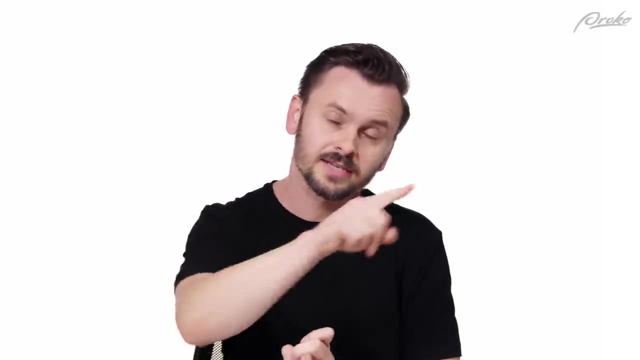 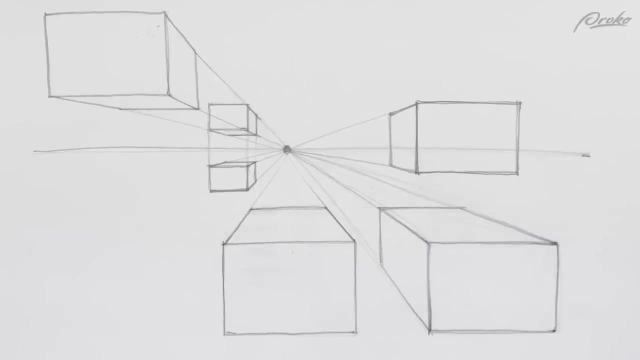 Could it be? Two point perspective. Stay tuned, Here's a warm up: draw boxes in one point perspective. I'm gonna give you guys a project in the next premium video, but for now let's do this as a warm up. Copy this page that I drew, then put it away and try to draw your own boxes in one point. 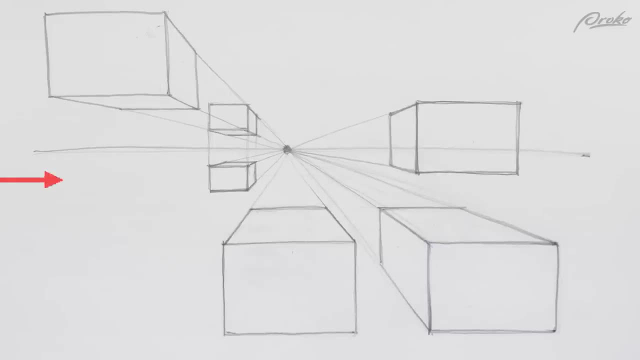 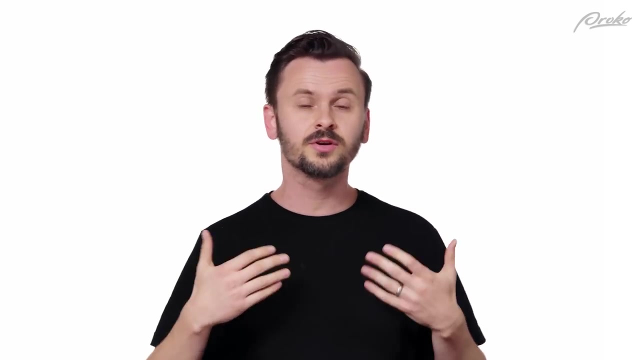 perspective. Draw these boxes going up and down and left and right and into the distance, Play with various proportions and dimensions. And remember this is a warm up. this is something you can repeat for five minutes before any of the upcoming perspective projects. 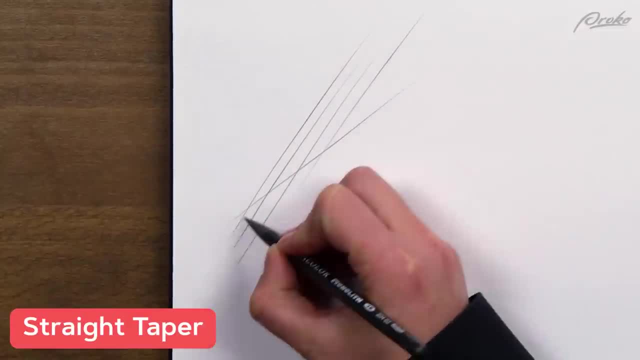 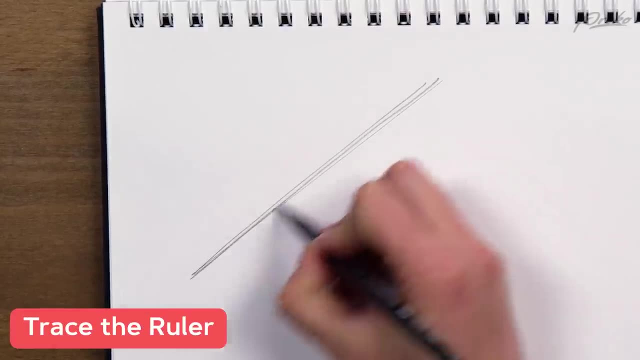 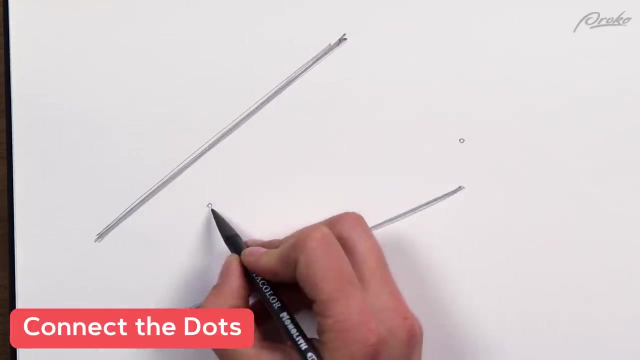 This is also a good time for me to remind you of all the warm ups I already showed you in the full course. that incorporated straight lines. There's a straight taper: trace the ruler and connect the dots. We're gonna be drawing a lot of straight lines in this perspective section, so keep practicing. 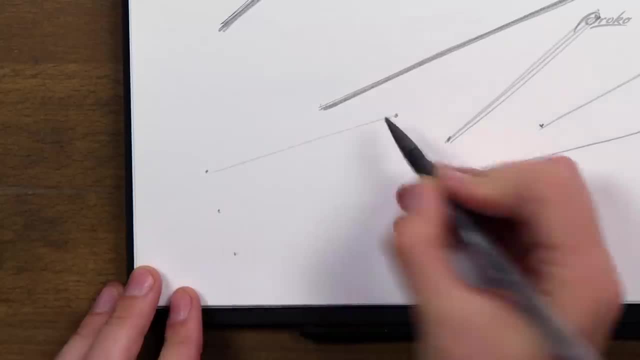 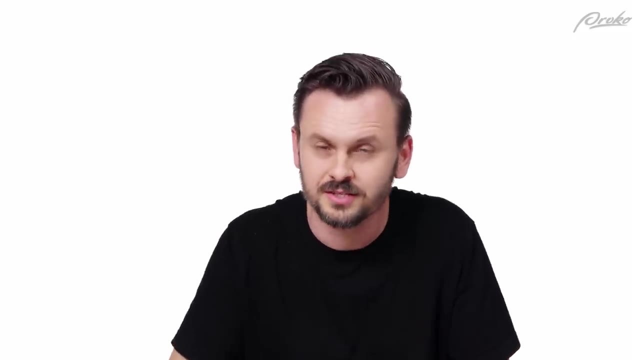 them daily, so that you're comfortable and you can focus on learning the concepts instead of struggling with your shaky hand. If you're finally ready, let's get started. If you're finally ready to get the premium version of the drawing basics course, that's. 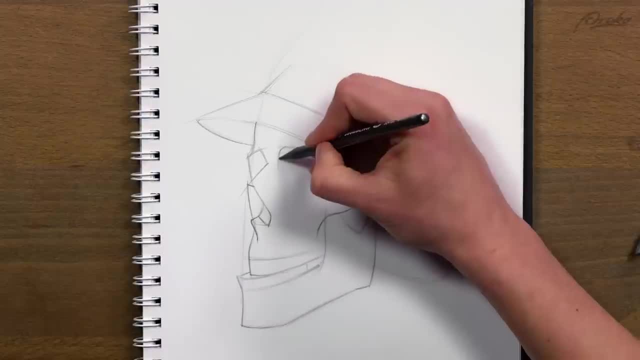 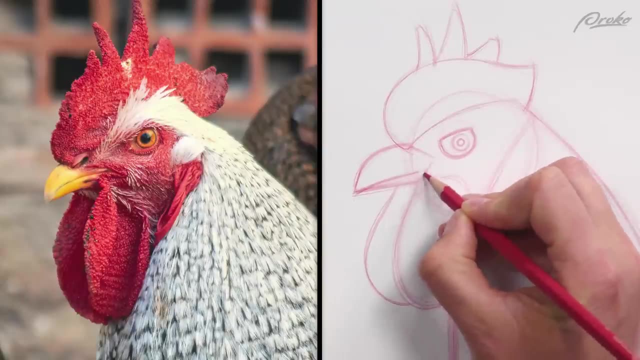 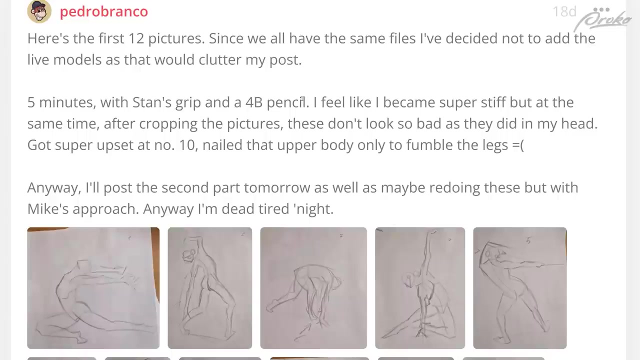 over at prokocom slash drawing. We've already learned how to control line weight with three different methods, how to develop confident line quality habits. We've covered shape, including accurate proportions, dynamic and interesting shapes, and how rhythms can help you draw better poses.